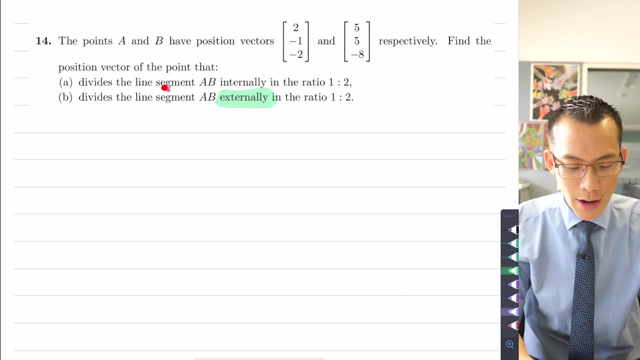 to part b here. I'm going to skip over part a. if you want to have a look at how to divide a line segment internally, just have a look at the previous example. but I'm just going to focus on this one, because number one it's quite different geometrically and number two it 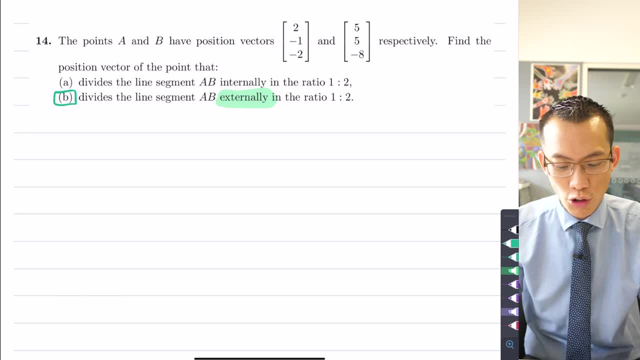 opens up a bunch of other questions that you need to think through in a fairly logical way, but thankfully they're consistent with what we've already established. so let's see if we understand what's going on here Before we get to the particular position vectors that we have. 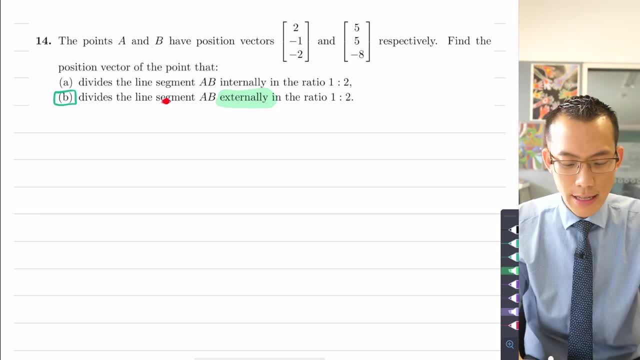 let's think about what. could it mean to divide a line segment externally? Well, if I were to provide for you some point a and some point b then to divide that line segment externally, I'm going to try line segment internally. don't know why I did that so thick. let's try that again to divide it. 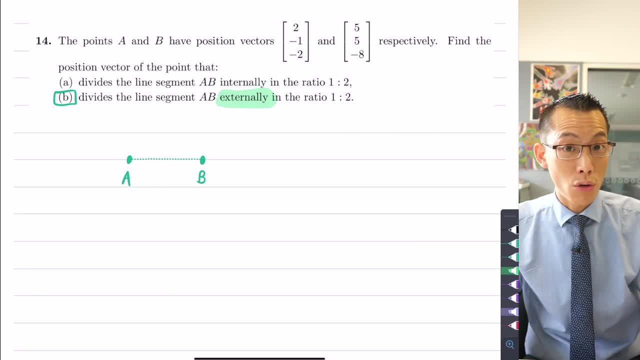 internally. the whole point is that some point- let's just call it p for point- some point p is going to be internal to this particular interval, this line segment. so if we were dividing- well, not if we're dividing in part one- it says divide it in the ratio one to two, then I would divide this: 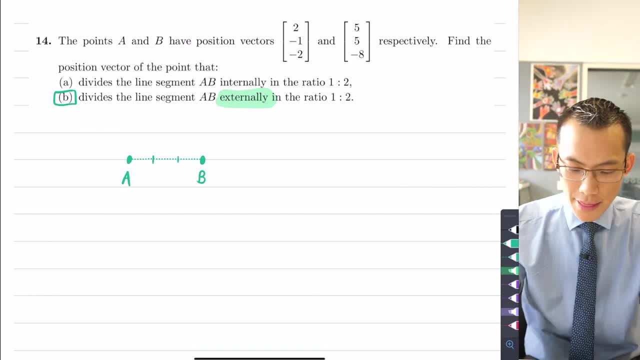 into, as we've seen before, three equal segments, and then p would be here to give me this ratio of one to 2.. So that's what internal ratio division looks like. Nothing too dramatic. We understand that P will be between A and B, It will be on the inside of A and B, and that's where 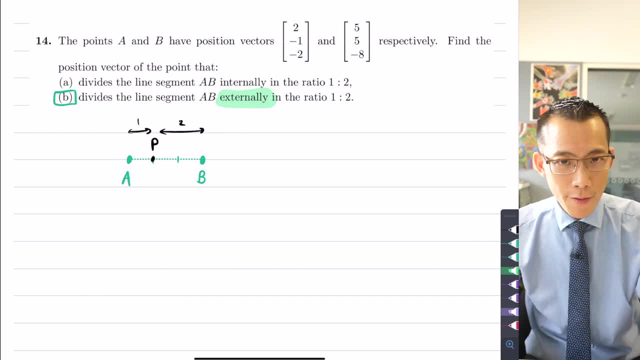 the internally word comes from Now. therefore, I hope the logic carries for you that if that's what internal division of a line segment is, then external division is on the same line. So what we can do is we can imagine this going off in opposite directions for infinity. but 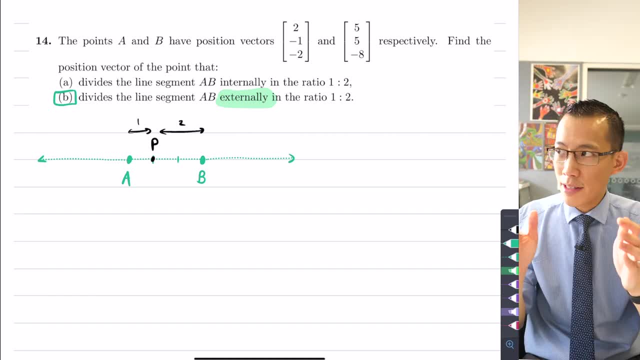 that point P is not going to be on the inside of A and B, It's going to be on the outside. So what I'm actually looking for, let's get rid of this particular one that I drew before. I don't need this divider either. What I'm looking for is some point out here or out. 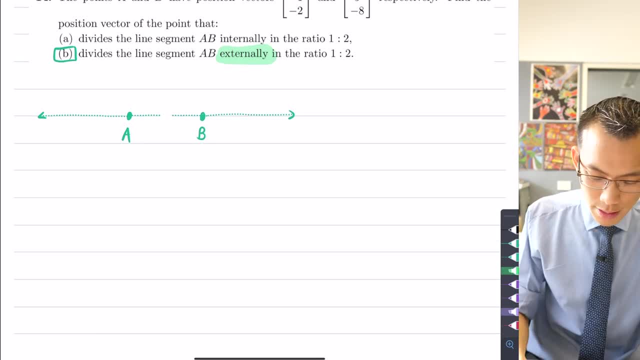 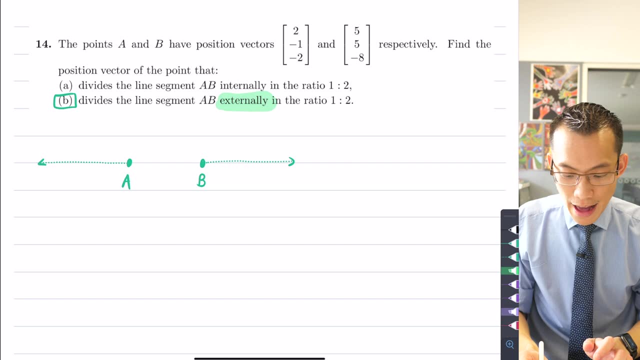 here. Maybe I'll highlight those. In fact, I can just get rid of this one there. This is where I want my point P to be. I need to find the place Somewhere along either of these two. we would call them rays, I guess, because they start. 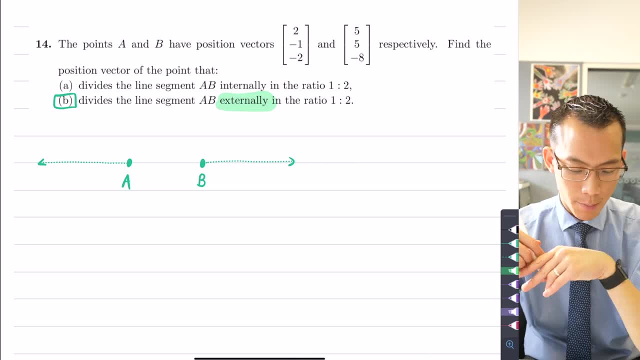 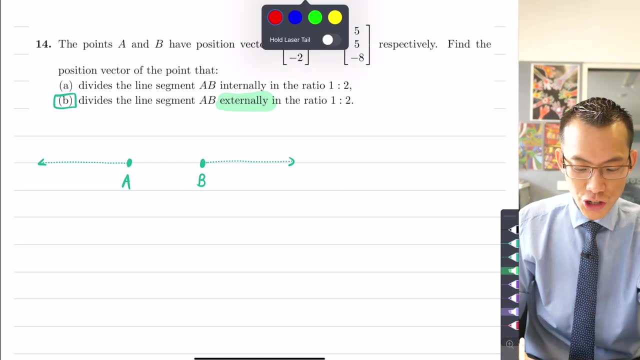 somewhere A and B and then they go off to infinity. We want to find the place along either of those rays where P could be. that will still have the same ratio, one to two- but it's different, It's going in different directions. 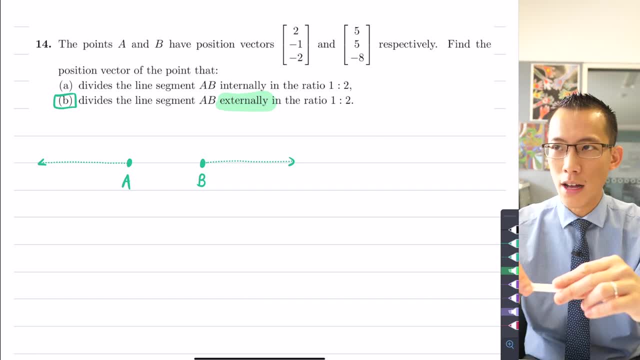 Now, some of you will have encountered a ratio division formula within quantum geometry in earlier years. You might have been extended into that And some of you will have learned that there's kind of a shortcut way, which I'm going to show you in just a moment, which 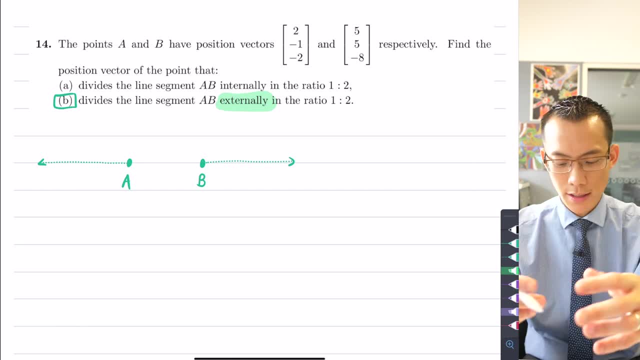 I'm going to deal with at the end of this question to be able to get to the answer. I'll get to the shortcut in a minute, but I actually want to make sure you understand why the shortcut works. So what would this actually look like? Well, I want you to call back If you were doing. 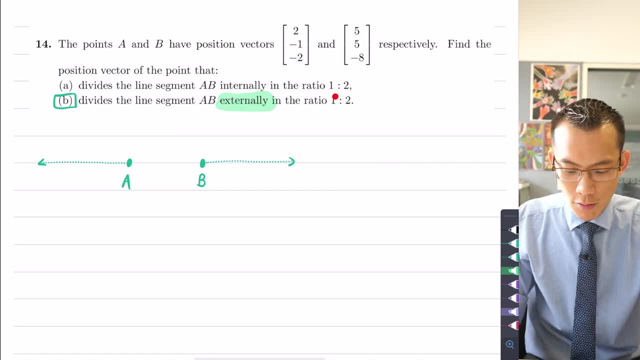 actually we'll just use this example here. If you're doing internal line division, right, We're dividing this interval AB, AB internally in the ratio one to two. Now, what this means is you can see, because I'm paying close attention to the order A. 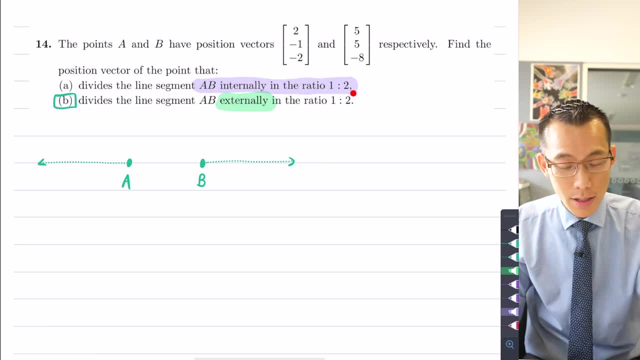 is first, B is second, one is first, two is second. The question I want to pose to you is: which of the points A and B, which point will my new point P be closer to? And if you remember from last example, we can say: well, since the ratio one out of the one to two, 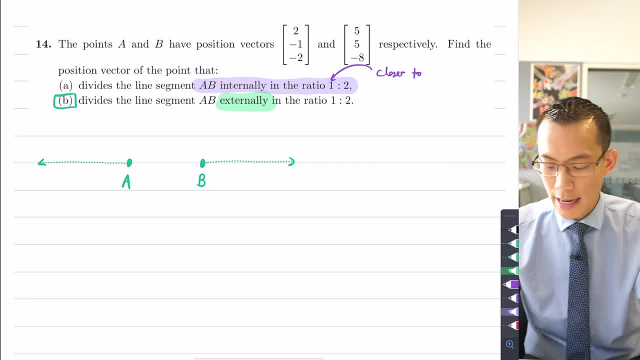 is smaller, I'm going to be closer to the first point than the second. that is, closer to A than B, right? If I are in the ratio two to one, then I'd be closer to the one, that's the B side rather than A. 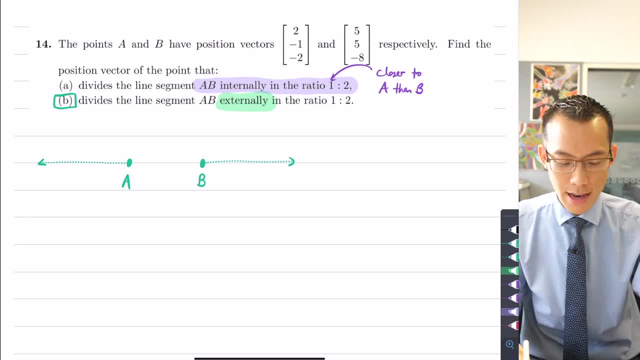 Now, thankfully, mercifully, the same kind of logic applies when we're talking about external divisions. So when I'm trying to divide this line, segment AB, externally in the ratio one to two, again I look at the order: A comes first, B comes second, the one. 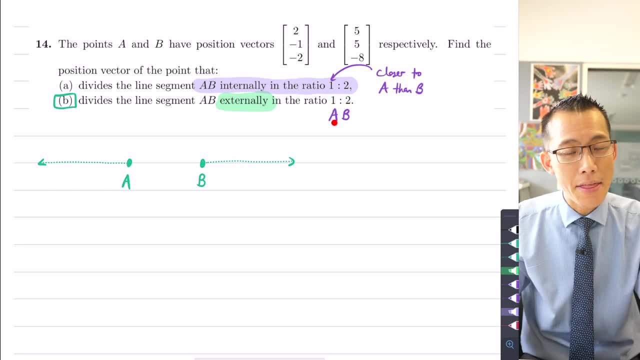 comes first, the two comes second. I'm going to be closer to A than I am to B. So when you have a think about which one of these rays I'm going to be on, which one of these rays is closer to A than to B, And the answer is, well, it's this left-hand one, It's the. 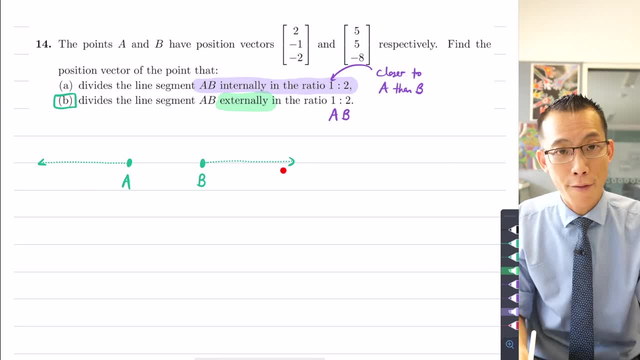 one coming out of A. If you picked any point over here along the ray from B, you would always be closer to B than to A, So you're not going to get the ratio one to two. You would get a different one. So we'll get to that different one later on, But for now what you need to 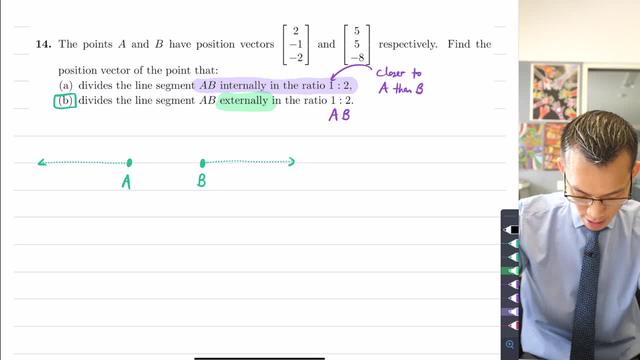 know is I'm looking for that point P that I'm going to position right about there, such that you get this ratio one to two, when instead of going, say like this, instead of going one to two, I now have to go outside of this interval AB, So instead of going in the same, 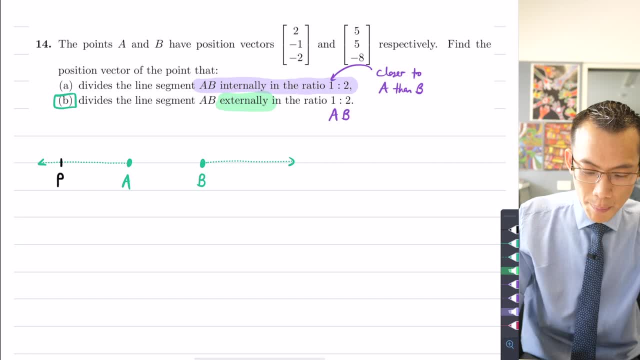 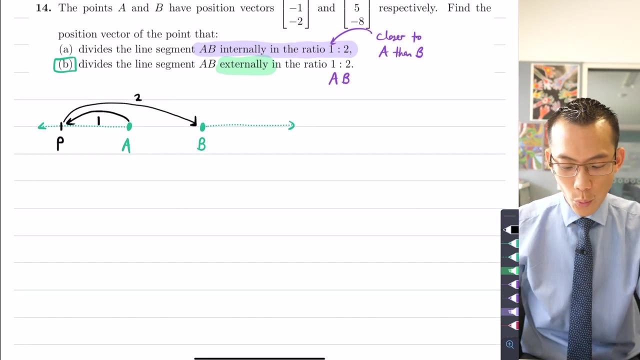 direction. I'm actually going to have to go first in the opposite direction, from A to P, That will be my one, And then I'm going to go from P over to B, That will be my two. So this is the one to two ratio that I'm after now, And, having found that we can now 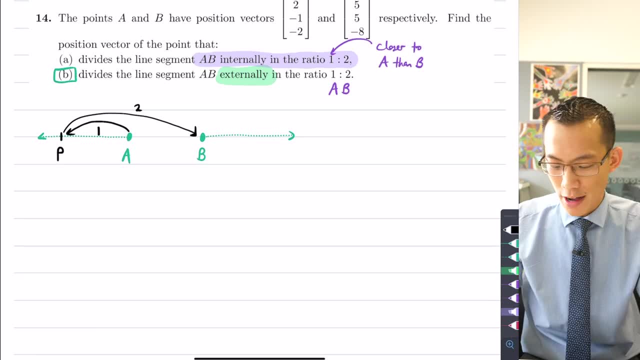 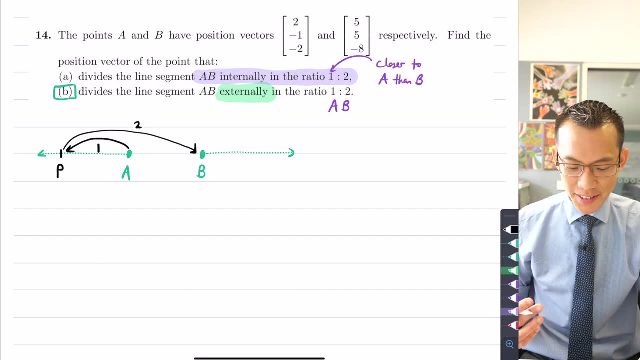 work out where P will be on the basis of geometry, And now I just need to crunch the numbers of this particular A and this particular B. All right, So now that you've got a handle on what external division means, let's go ahead and try and find this answer. This is part B that we went straight to In order. 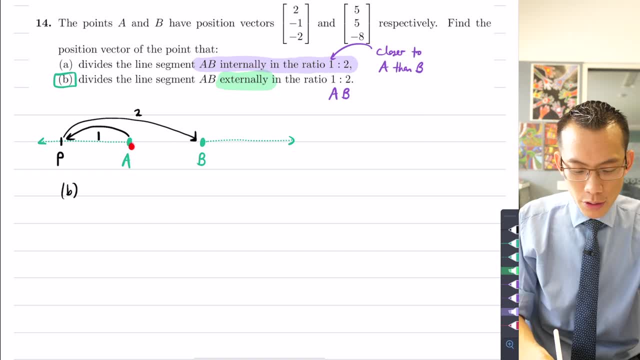 to find where this is. hopefully you can see that in order to get from A to P, it's backwards to going from A to B. So in fact I just need to find this. AP vector is just the opposite of the AB vector: Same magnitude, opposite direction. So in order to find out what AP, 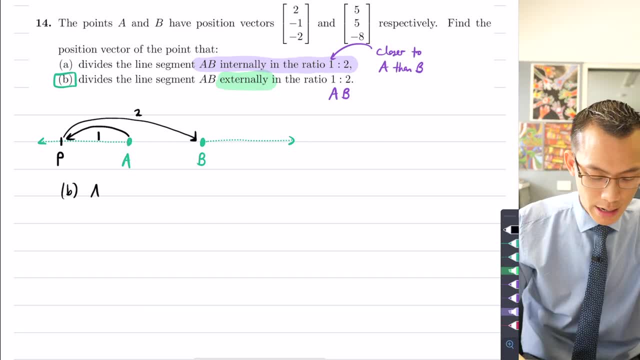 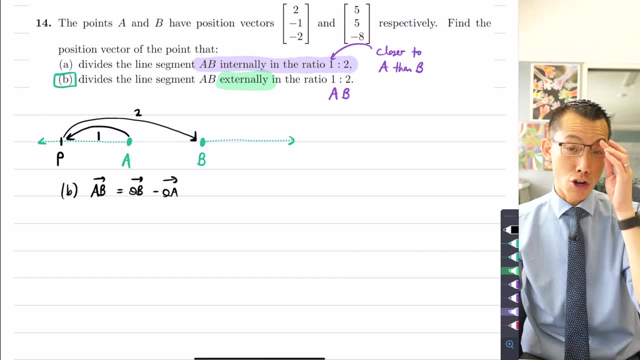 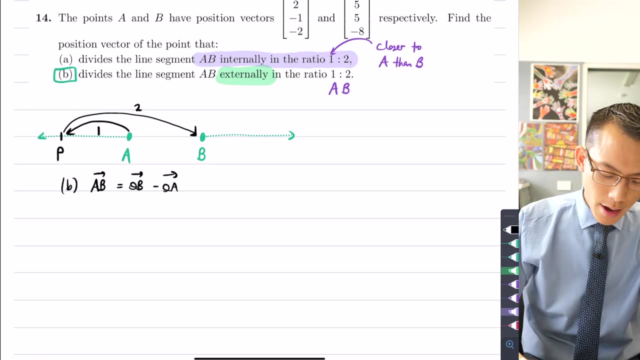 is. first I need to find out what AB is. So let's go ahead and do that. AB is equal to OB. take away OA And I've explained the geometry and the relationship between the sides of a triangle to get to that pair of vectors. What is OB or what are OB and OA? 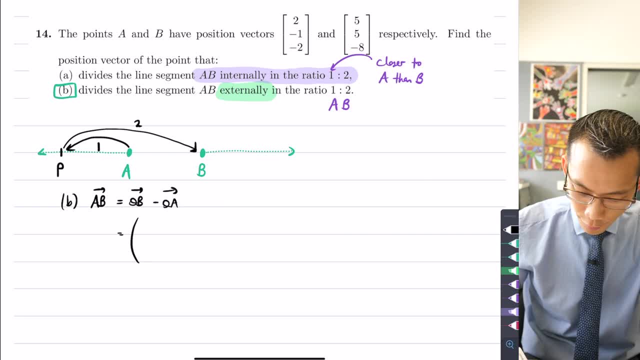 I'm going to get. I'm going to put this all into one step. I'm going to get five, five and negative eight from OB, And then what I'm going to do is I'm going to subtract, subtract all of these, So that gives me minus two plus one plus two. You're noting that. 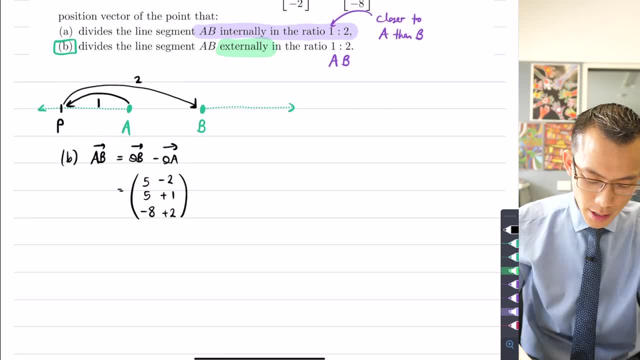 I've flipped around the signs of the negative one, the negative two, because I'm subtracting. What's that going to give us? Well, it looks to me like I'm getting three and then six and then negative six. So maybe just double check those signs. Looks good, So that's AB. 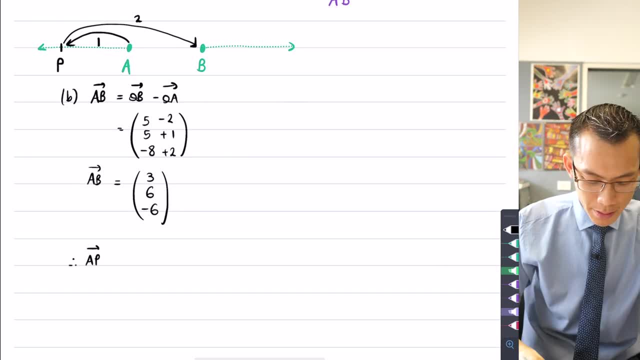 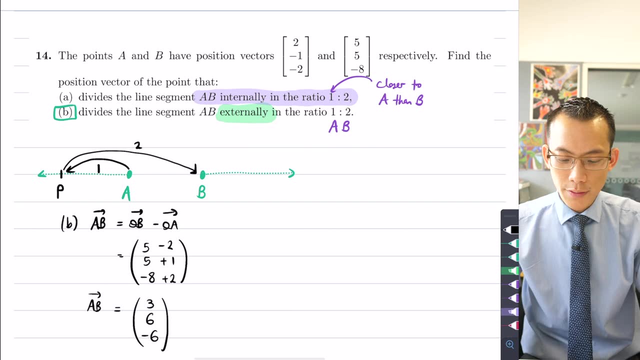 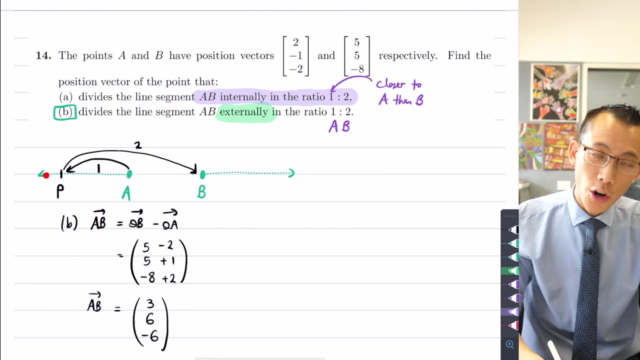 So therefore I can say AP will be the opposite of that. So I guess that would be negative three, Negative six and then positive six. And because what I'm looking for is the coordinates of P, the way to get to P directly is from some origin to A first and then go over to P In. 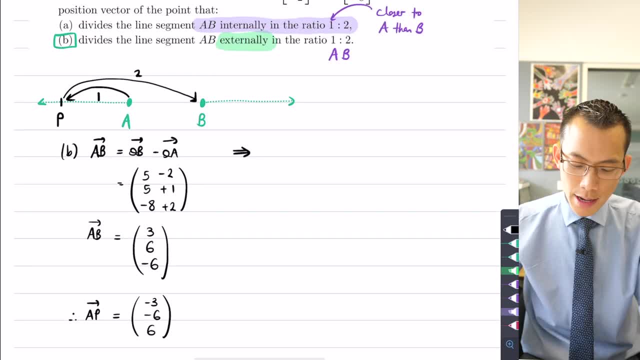 other words, I'm just going to put it here. What this implies is that OP starts from O, goes to A first and then goes from A over to P, because I know what each of those vectors is. I've got OA up the top there. two negative. 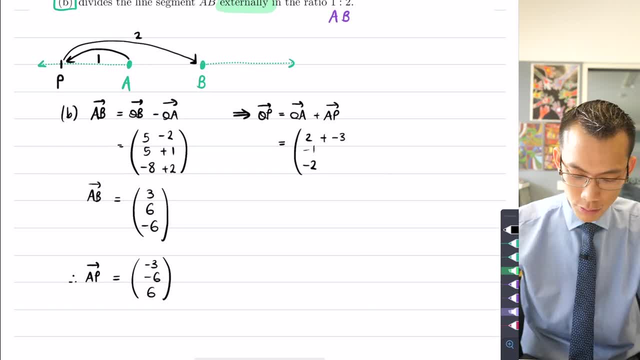 one negative two, and then I'm going to add this negative six, and then I'm going to add six. So what do I get here? Two minus three is negative. one Minus one minus six is negative seven, And then I'm going to get a positive four down the end. That's OP which. 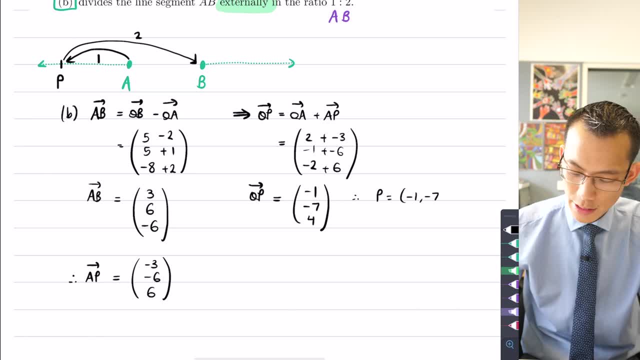 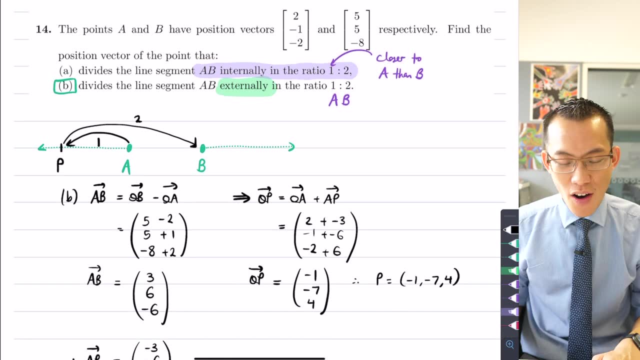 means, therefore, that P has the coordinates negative one, negative seven and then four. Okay, So that's how to do the external division of a line segment. It is a bit weird because you've got to think about this whole going outside business rather than going inside. 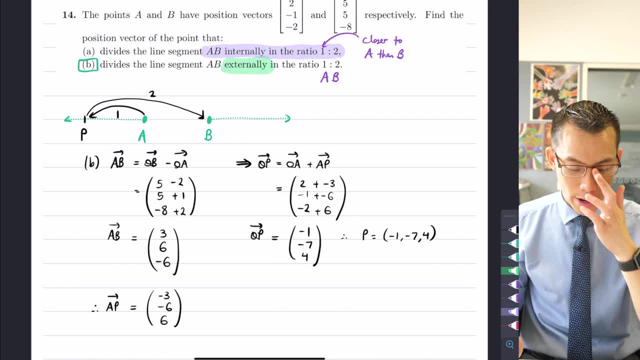 the interval. But this leads to that shortcut. by the way, You can actually use a ratio division formula if you've learnt one. I'm not a fan, as you guys know, of learning formulas without knowing why they work, but if you have a think about what is happening geometrically here, 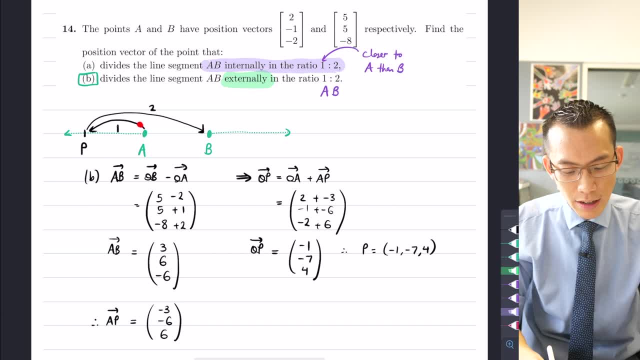 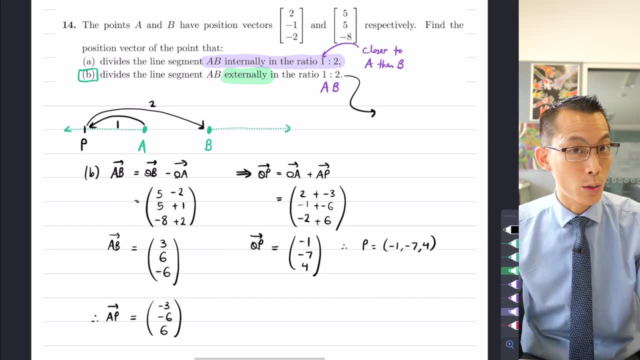 another way that you can do this is just to say: well, this is the same as doing negative one, because I'm going backwards, as it were, and then positive two. so if you learn a ratio division formula- and some textbooks will provide it for you- you 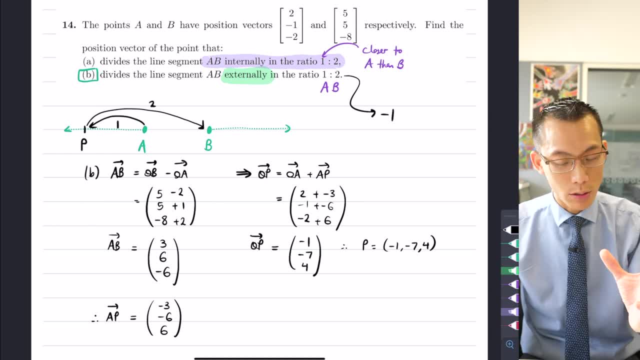 can just simply say it's the same as doing a regular internal division, but just making the ratio one of the numbers negative. in this case the negative one makes the most sense because that's going backwards and then forwards in the original direction. so that will give it to you. but I also think it is really 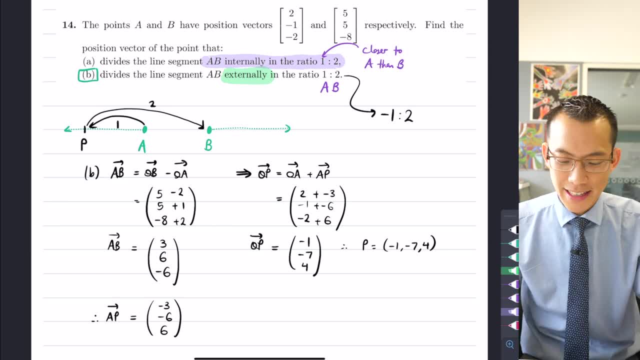 important to know why it is that that works now. lastly, I do want to talk about- it's not addressed in one of these questions here, but I want to give an example of what it looks like to divide this line segment externally still, but where the ratio is opposite. so suppose let's just call this part C, if I can. 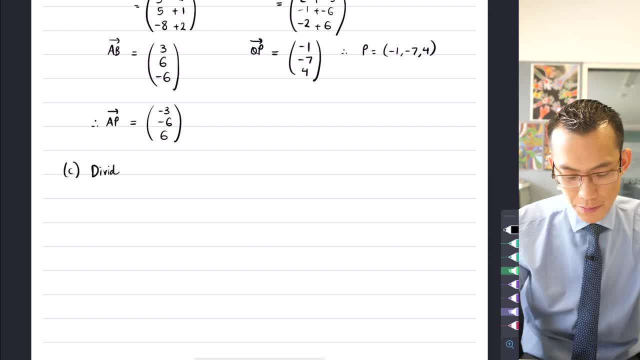 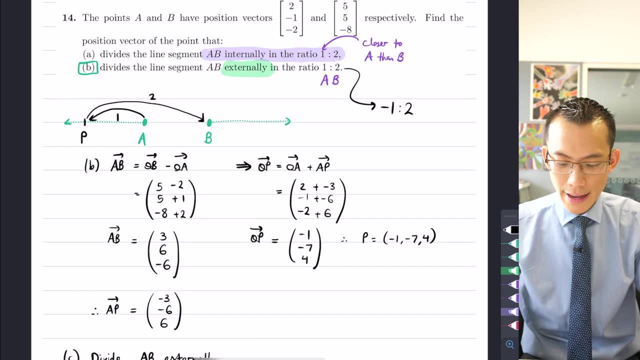 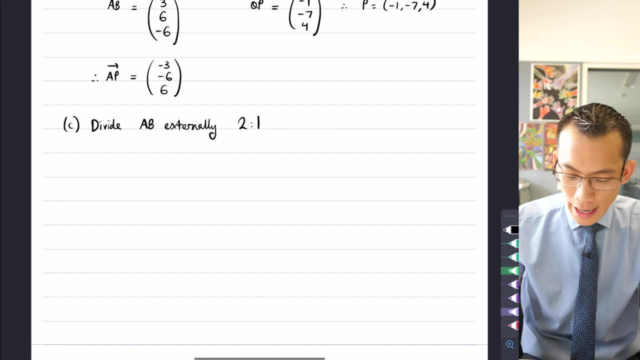 write that if we divide a- B externally. that needs to be said. and instead of going, as was asked here, one to two, what if we went two to one right? two to one would mean, when I again pair up this particular interval, a B, in that order with the: 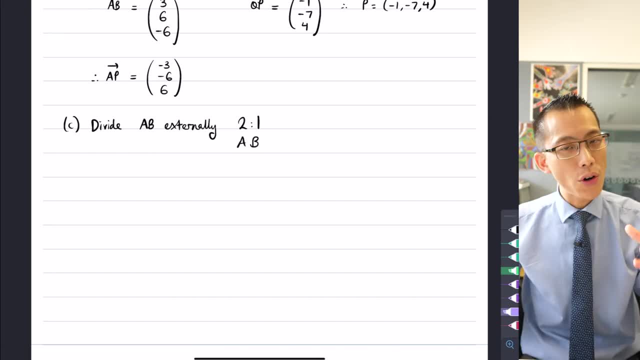 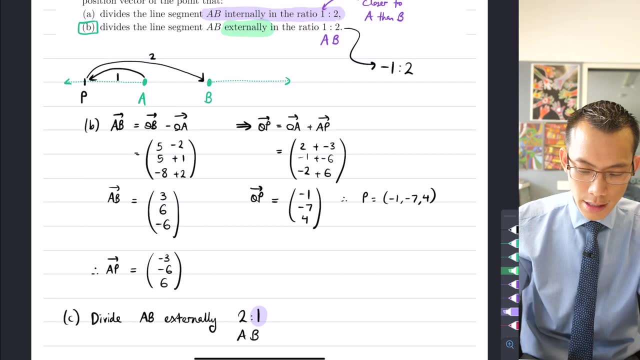 ratio a and B, you can clearly see which of those two points you're going to be closer to. the one is smaller, so therefore you're going to be closer to B than to a. so, if I go back to my diagram up here, let's just grab this whole thing. 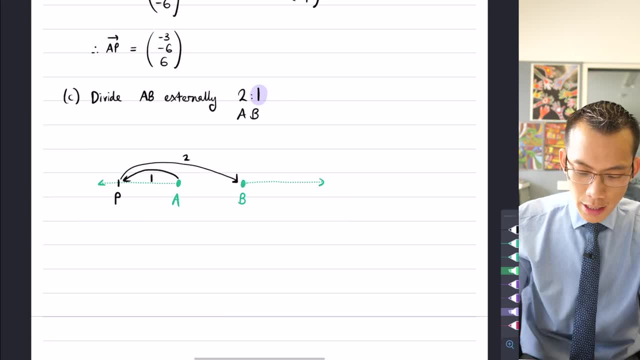 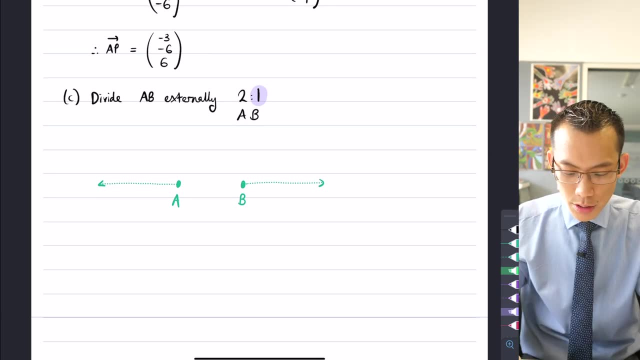 and I'll delete off the parts I don't need. so here is my a- B situation and I'm wondering where will PB be in this case? I need to be closer to B than I was today. I'm going to be on this ray rather than the other one. the two to one comes from. 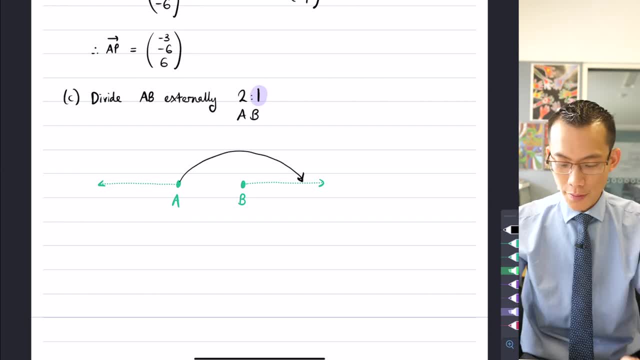 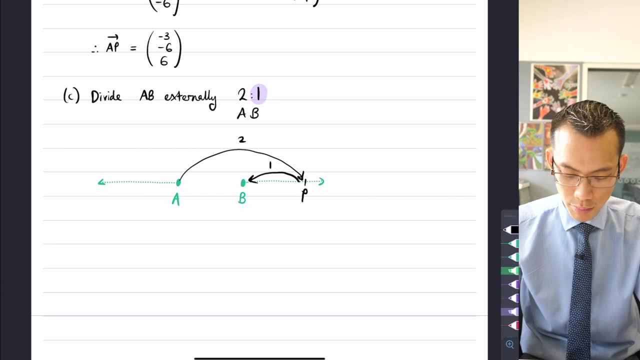 starting from a and going all the way over in the big jump. first we'll call that P, that's going to be the two, and then the one comes in the opposite direction, like: so I should put that one underneath just to be a little clearer, right? so in this case, once you find a, B, you're still going to need to do that. 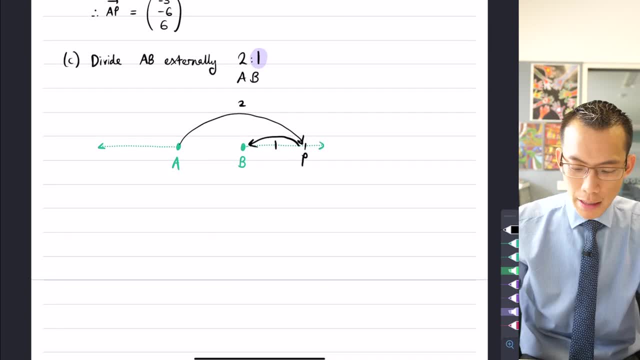 what is the most sensible way to get to P? well, because P is over here, it's closer to B. it would stand to reason that the easiest way to get O P would be to start at B, get from the origin to B and then go from B. 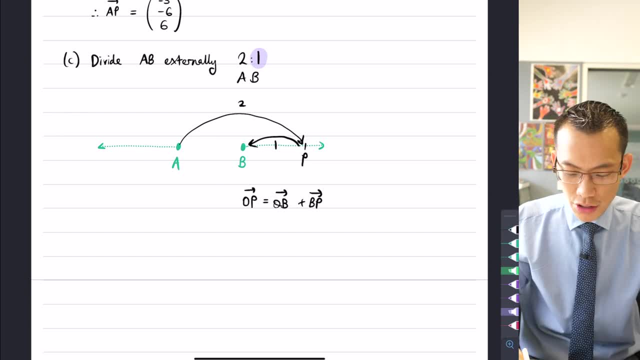 to P. however, in this particular one, because the ratio is two to one. that means that if I just grab this color here, hopefully you can see that B- P. if I were to go from here to here, it's the same direction and the same magnitude as going from A to B, it's just a different. 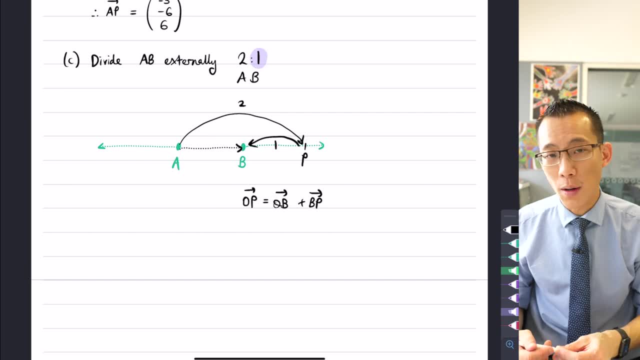 displacement vector. it's starting. the tail is starting in a different spot, starting at B instead of starting at A. so therefore, if this is a B, then it stands to reason that this is also a B, same direction and same magnitude. so therefore, to find out where P is, you just go OB and then you'd add AB, because